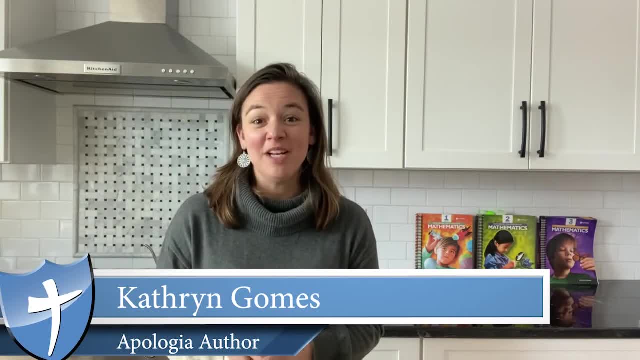 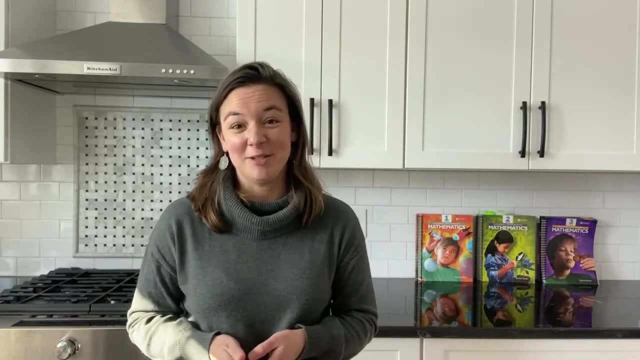 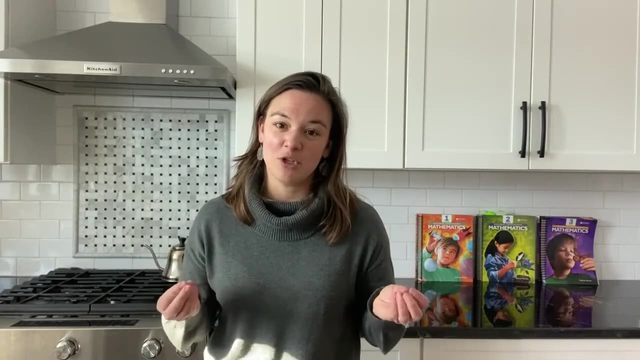 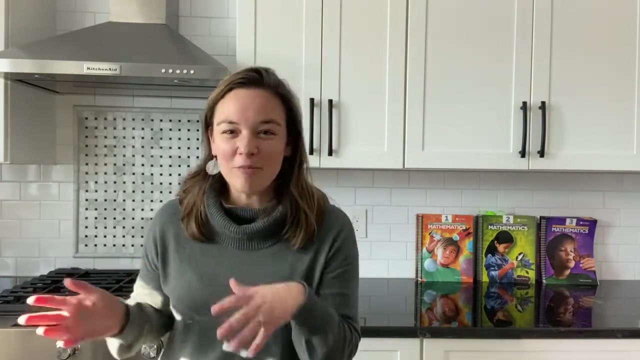 Hi, my name is Katherine Gomes and I'm the author of Exploring Creation with Mathematics, the brand new elementary math series for homeschoolers from Apologia. There's a well-researched progression that has just been shown to be a great way to teach students elementary math. That progression is concrete, pictorial, abstract. So all that means in sort of layman's terms is when you first introduce a new math idea to kids, you do it concrete. 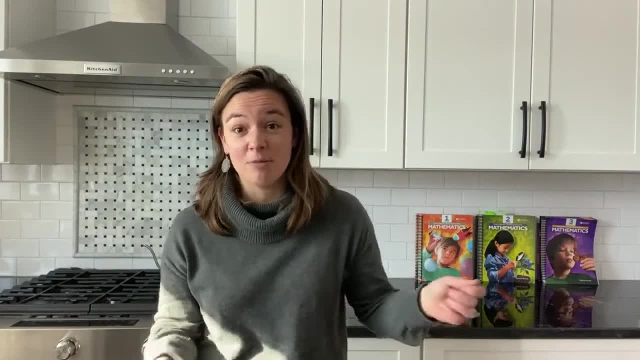 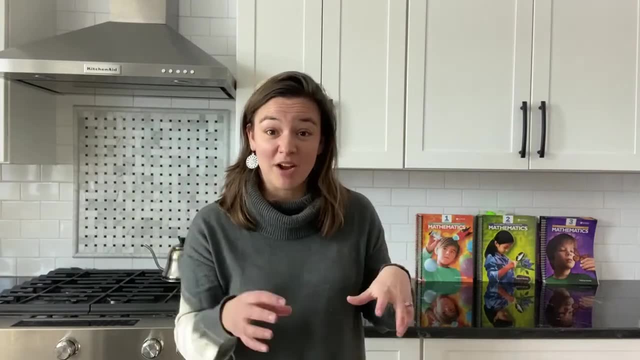 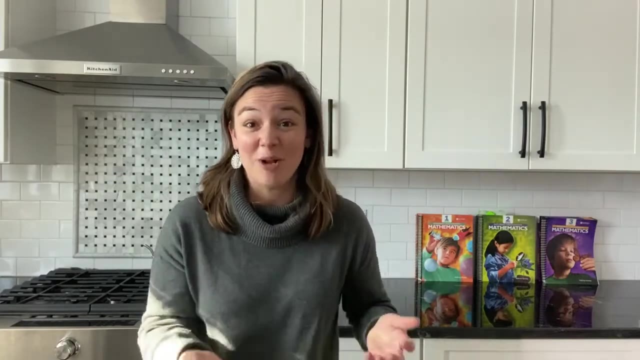 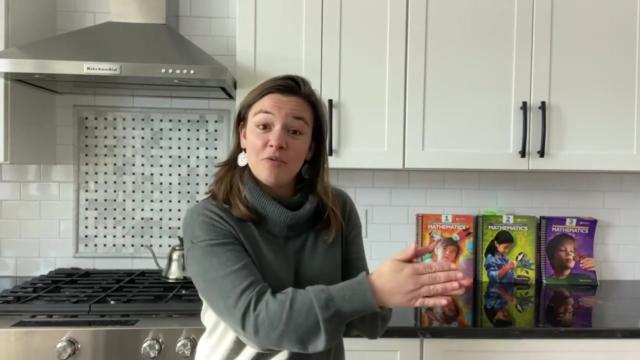 So you start concretely. You're going to use beans or monopoly money when you're teaching long division or fraction tiles so that kids can touch and feel and move things around. And a lot of times the objects that I use in the books are household items that kids are familiar with or that they even play with when they're not doing math. So you start concretely, then you move to pictures and drawings of those math ideas using those objects. So now we're on the page but kids are drawing and they're still able to visualize. 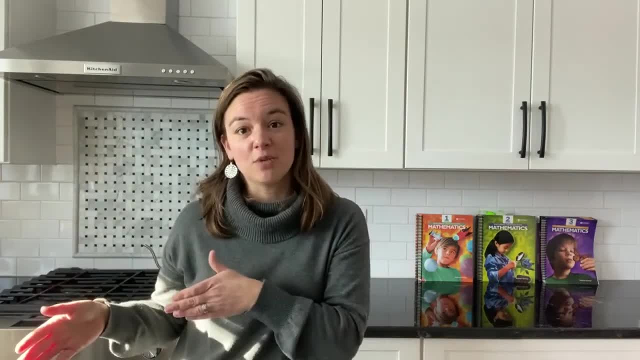 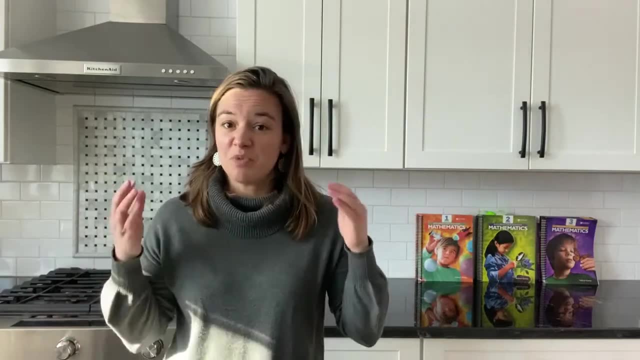 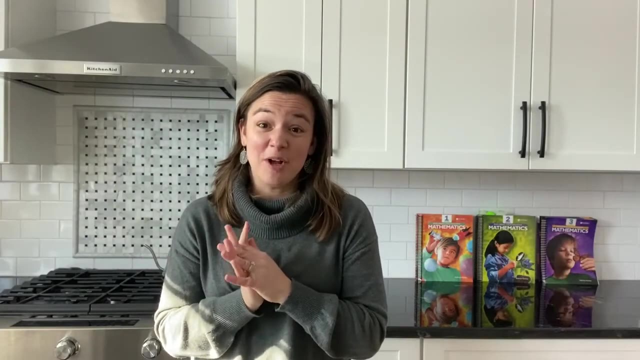 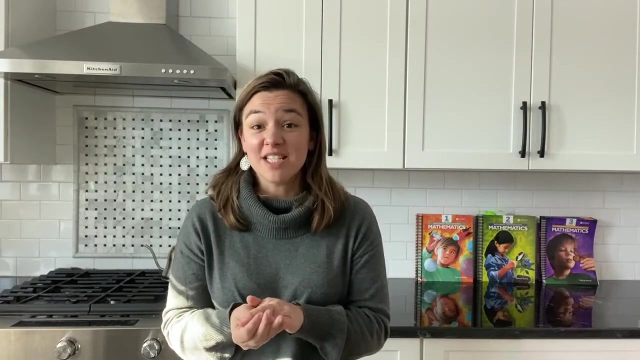 And then finally we move to abstract, where they're going to learn the long division symbol or they're going to actually add fractions. Moving kids through those progressions just really helps them master the idea. I know there's a lot of different choices out there for elementary math and it can be difficult to sort through. So there's two things I think really make this series unique. First, it does have a Christian element to it. 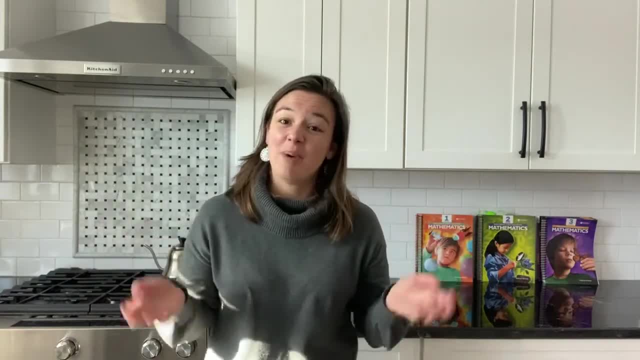 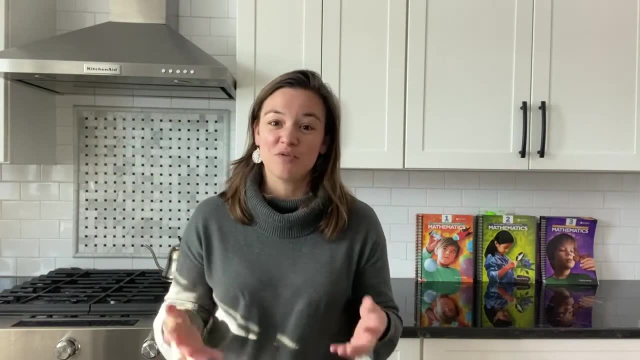 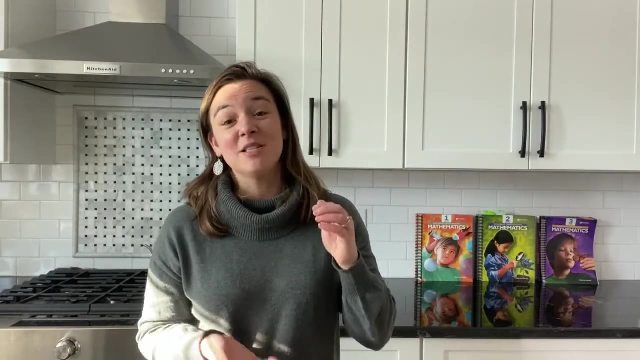 I was so excited to pour my faith and my family. I had a passion for how learning about math can teach us more about the Creator, And so at the beginning of every unit, I've written a short devotional that helps the kids see more of God in what we're learning about math. There's so much we can learn about His beauty and His truth and just His creation, as we're exploring mathematics. 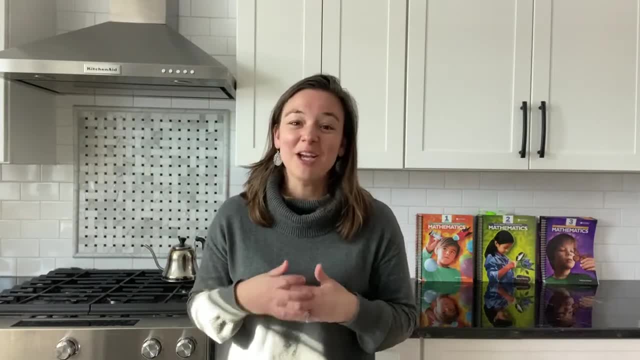 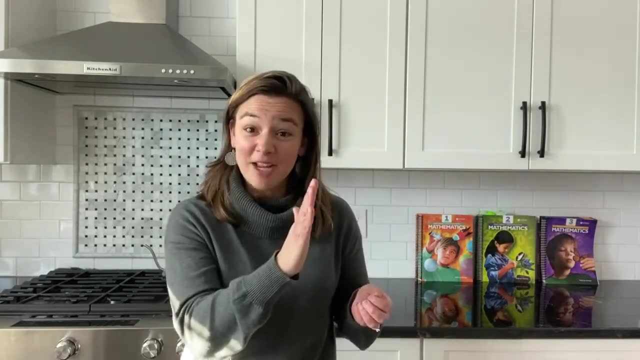 So I think you'll love the program because we really put a lot of time and energy into making it so easy and painless for you the parent, you the parent- whether it was putting a thumbnail on the answer key so you could just check the answers at a glance, or giving you a complete list of every little household item.